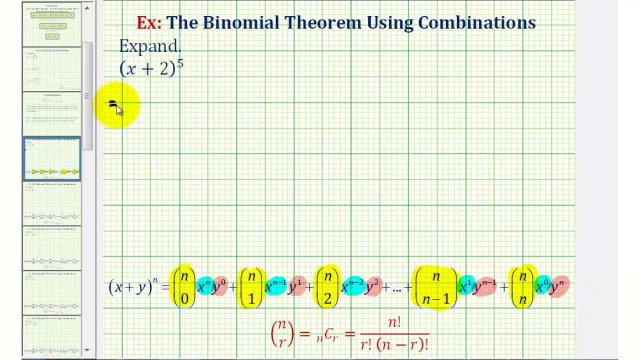 So let's go ahead and expand our binomial. The first term would have a combination of five choose zero, and we'll have five factors of x and zero factors of two. Next term, we'll have five choose one as our combination and we'll lose a factor of x. 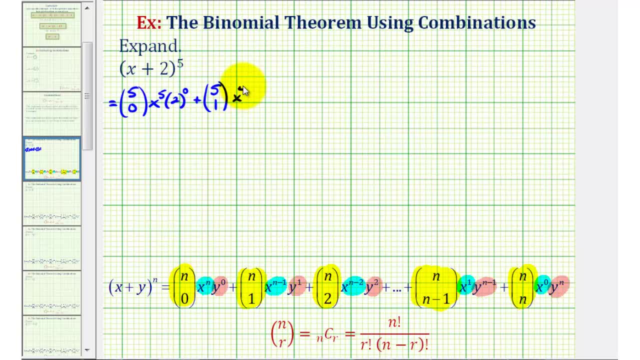 and pick up a factor of two. So we'll have x to the fourth, Two to the first, plus next term would be five. choose two times x to the third, two to the second. Again, notice how these exponents always add to five, which is our original exponent. 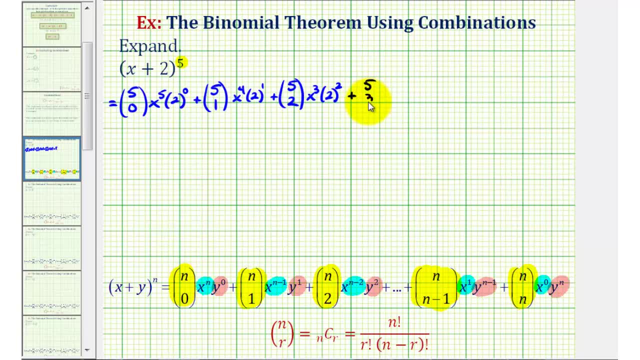 And now we're going to have five choose three, and we'll have two factors of x and three factors of two, plus five choose four. We'll have one factor of x and four factors of two. We have one more term: five choose five. 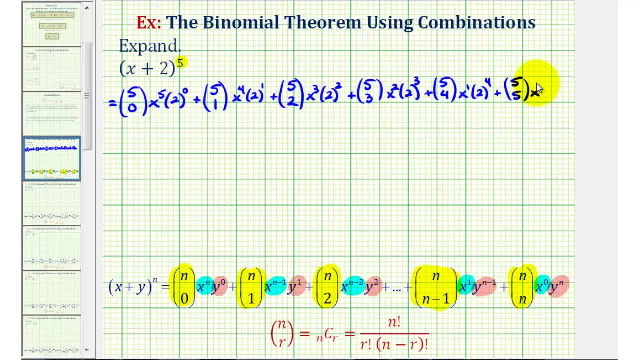 So we know we're done and we'll have zero factors of x and five factors of two. Now we've applied the binomial theorem. we just need to simplify this to find our expansion. There is a way to evaluate these combinations using Pascal's triangle, but for this example, 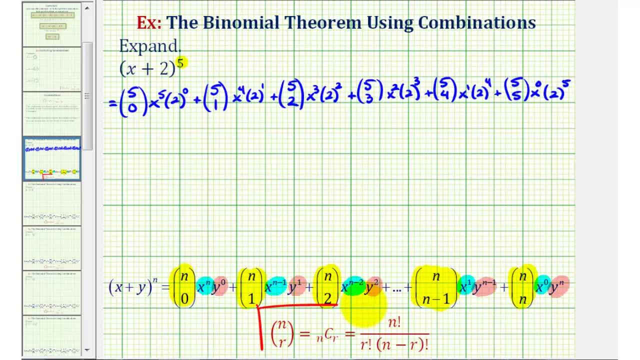 we're going to go ahead and use the equation, We're going to go ahead and use the factorial definition of a combination given here. So for five, choose zero. we would have five factorial divided by zero factorial times five minus zero factorial, which is just five factorial. 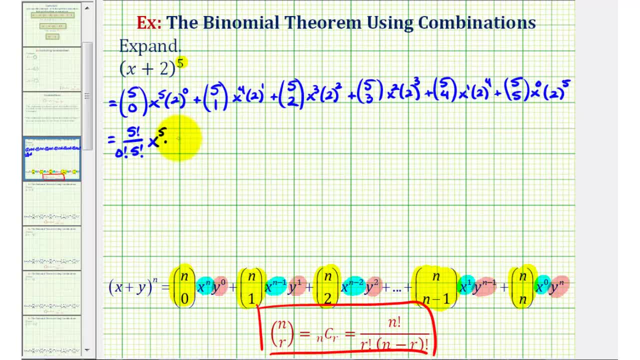 We have x to the fifth and two to the zero. is equal to one plus five. choose one. is equal to five. factorial divided by one. factorial Four. factorial x to the fourth times one factor of two plus five. choose two. 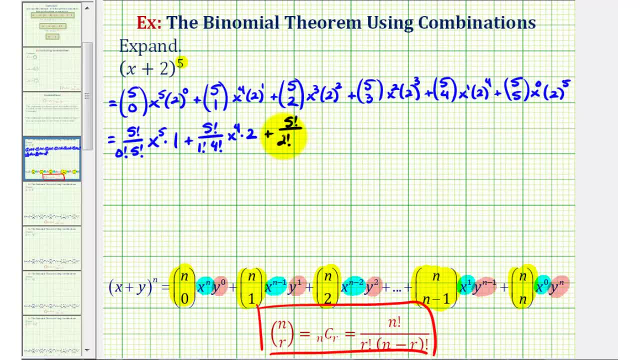 that would be five factorial divided by two factorial, three factorial x to the third, two to the second. that's equal to four plus five. choose three, that would be five factorial divided by three factorial: two factorial x to the second, two to the third. 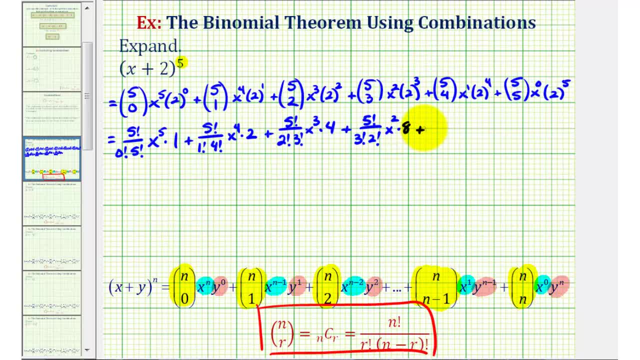 is equal to eight. so we have times eight plus five choose four. that would be five factorial. divided by four factorial. one factorial x to the first, two to the fourth is equal to 16.. Last term we have five choose five. that would be five factorial. 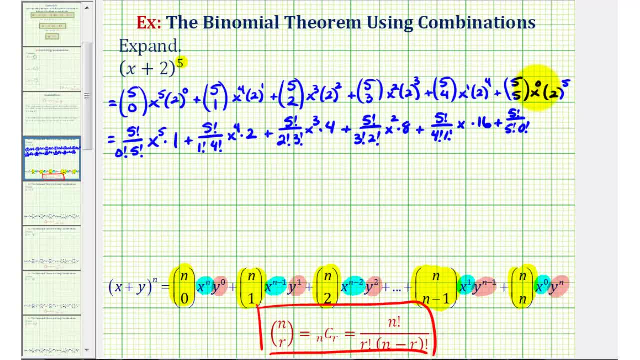 divided by five factorial zero. factorial x to the zero is equal to one. two to the fifth is equal to 32.. Now we'll continue to solve this problem, We'll continue simplifying. Well, five factorial over five factorial is equal to one zero factorial is equal to one. 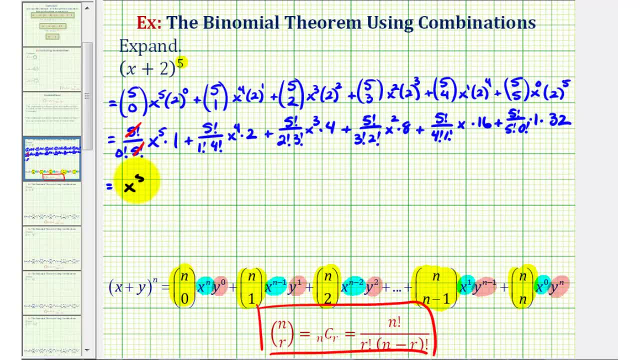 so notice how this first term would just be x to the fifth. If we look at these fractions involving factorials, several of them are equal to each other. Notice how this fraction here is equivalent to this fraction here. This fraction here is equivalent to this fraction here and this fraction here. 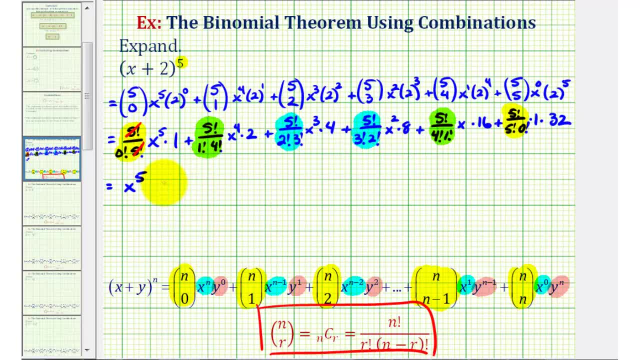 is equivalent to this fraction here. So for this next term, to simplify this, we'll go ahead and show the work. We have five factorial divided by one factorial, four factorial. Remember, we can write five factorial as five times four factorial. 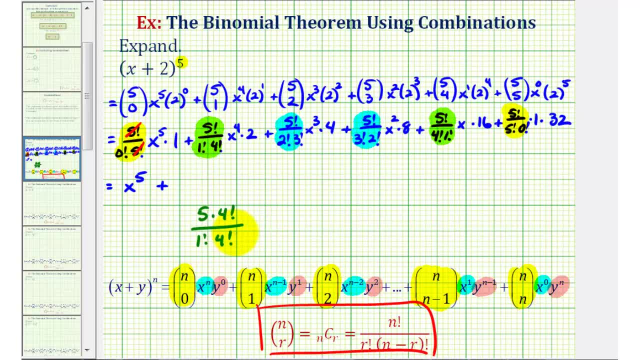 all over one factorial times four factorial. Well, four factorial over four factorial is equal to one. so this simplifies nicely to five. So if this is equal to five, we have five times two, That's ten x to the fourth, plus now we have five factorial divided. 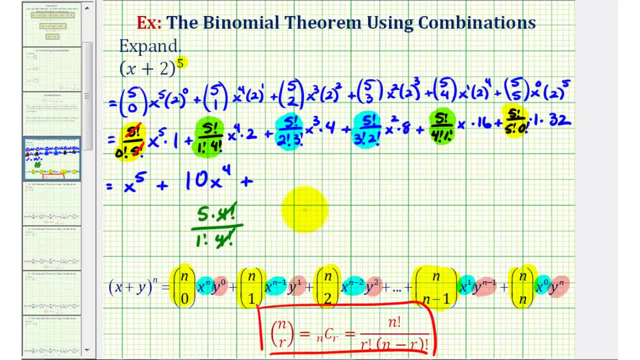 by two factorial, three factorial. So we can write five factorial as five times four times three factorial divided by two factorial, three factorial. This simplifies to one: two factorial is equal to two. twenty divided by two is equal to ten. 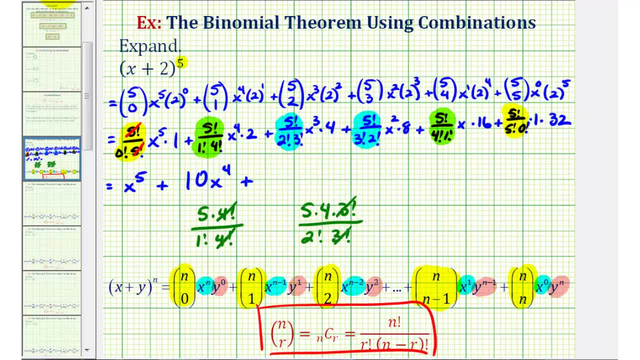 So we have ten times four, That's forty x to the third, For the third term. now remember, these two fractions involving the factorials are equivalent. So if this is equal to ten, we'd have ten times eight, That's eighty times x to the second.